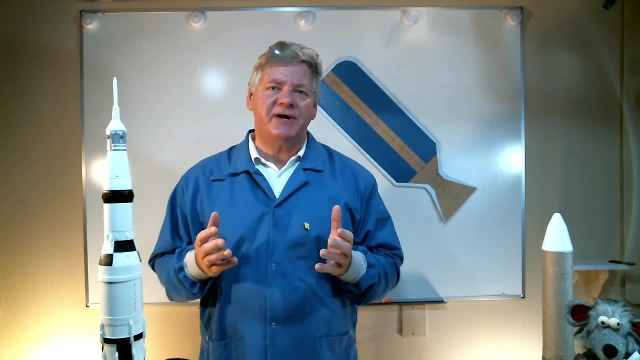 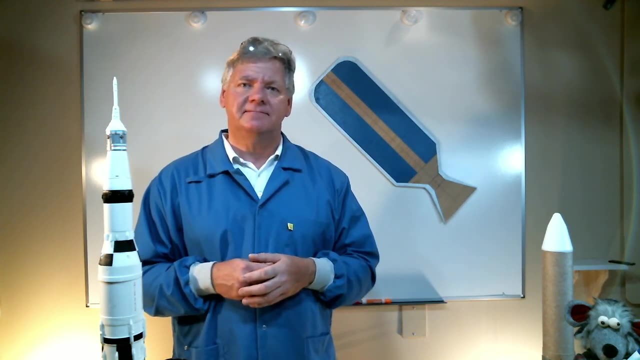 get the high-pressure gas inside the rocket motor? Well, the answer to that question is combustion. It's the chemical reaction that converts a solid or liquid fuel into a high-pressure gas. Let's take a quick look at the combustion process Now. there are three things that are needed for. 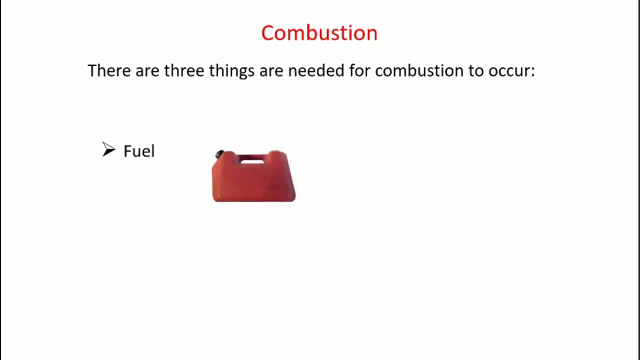 combustion to occur, First we need some sort of fuel, Second, we need oxygen And finally, we need a heat source to get the reaction going. Now, if any one of these three things is absent, the combustion process will never start, Or if it started and one of these is taken away. 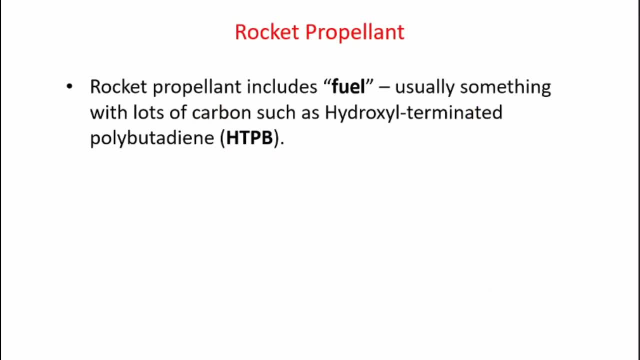 the combustion process will actually stop. Now let's take a look at rocket propellant. Rocket propellant includes fuel, usually something with lots of carbon, such as hydroxyl terminated polybutadiene or HTPB, to the rocket world. Now rocket propellant also includes its 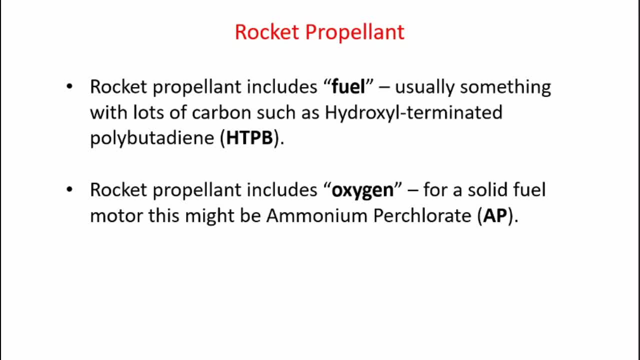 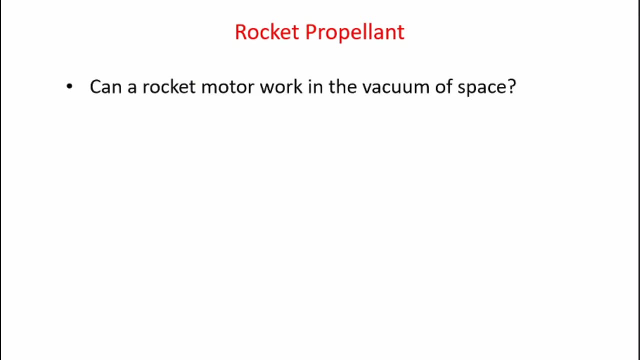 own oxygen. For a solid-fueled rocket motor, this might be ammonium perchlorate, which is known as AP. Now, if oxygen is built into the propellant, it doesn't need any oxygen from the outside atmosphere. So, with that said, can a rocket motor work in the? 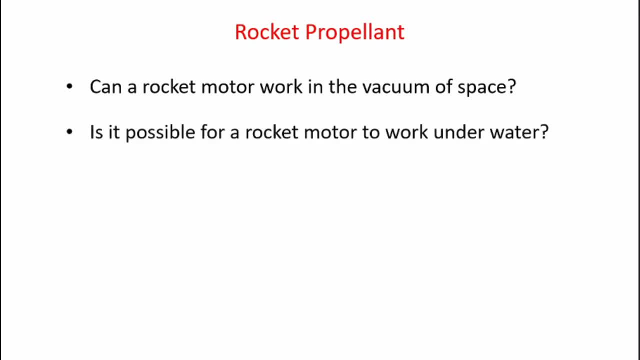 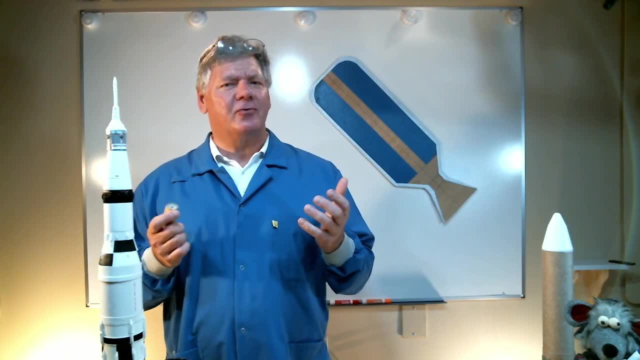 vacuum of space, Or is it possible for a rocket motor to work underwater? Now, the answer to both these questions is yes. So do we need proof that a rocket motor can actually work underwater? Well, let's do a simple experiment using a model rocket. 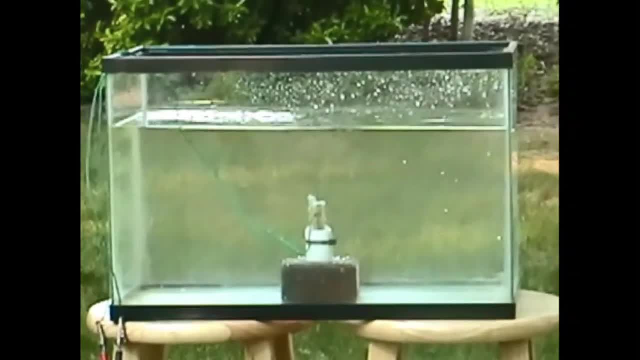 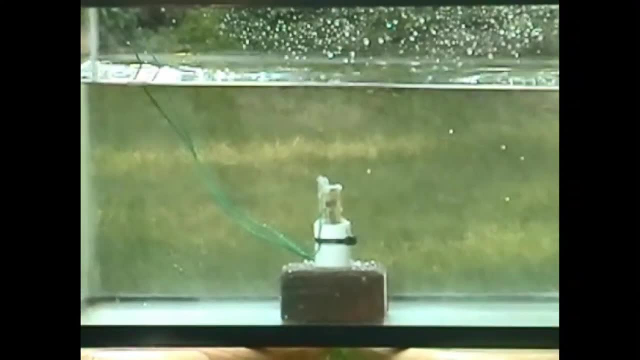 motor to see if we can actually get it to burn underwater. Here's my test setup: an aquarium full of water with a rocket motor inside. Now I have the rocket motor sealed with wax so the water can't get to the propellant before ignition. There we 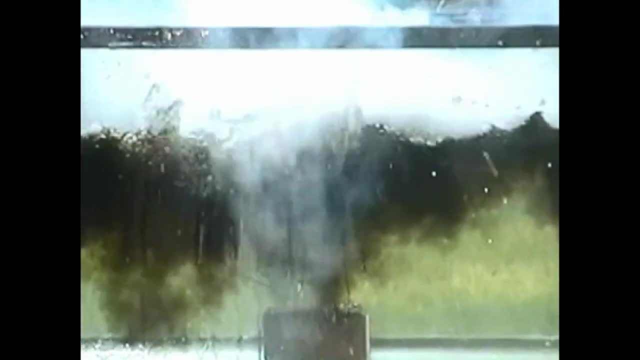 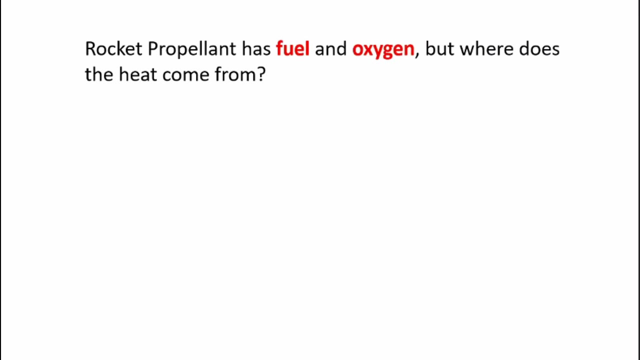 go, we see flame, so the rocket motor is actually burning underwater. So I said earlier, a rocket propellant had its own fuel and oxygen, two of the items needed for combustion to occur. But we don't have enough fuel to get the propellant to work underwater, So we need 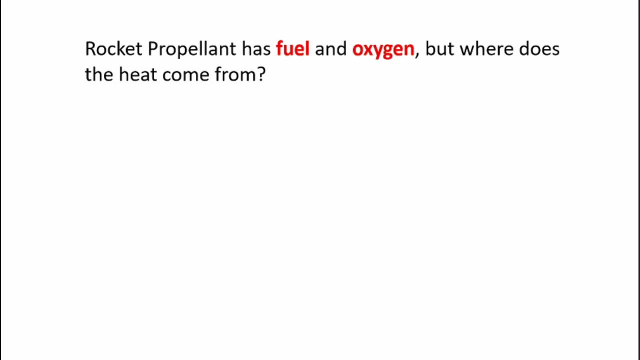 to get the rocket motor to work underwater. But where does the third item come from? Where does the heat come from? Now, the initial heat to get the chemical reaction started is supplied by the igniter. The igniter burns, ignites the propellant, and once that happens, 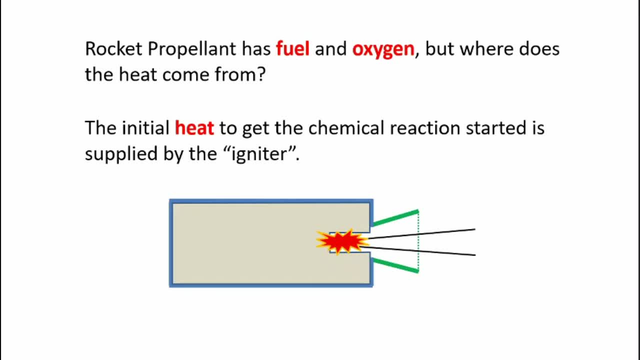 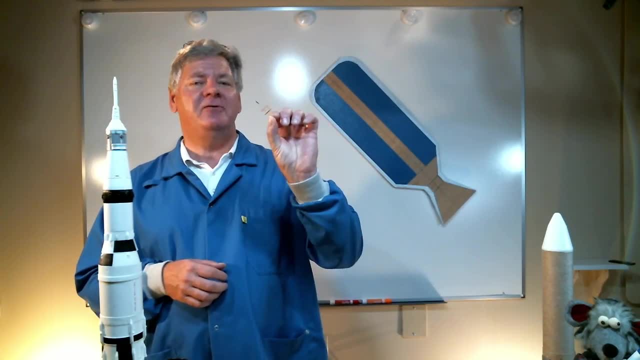 the chemical reaction is a self-sustaining reaction, and thus the motor propellant will continue to burn. Now let's take a look at a model rocket igniter. I have one right here in my hand. you can probably barely see it Now. this igniter works almost the same way. 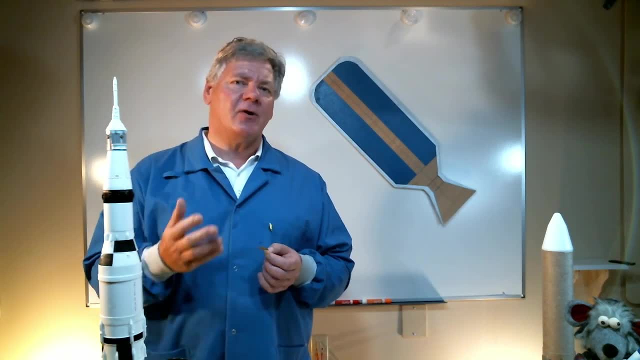 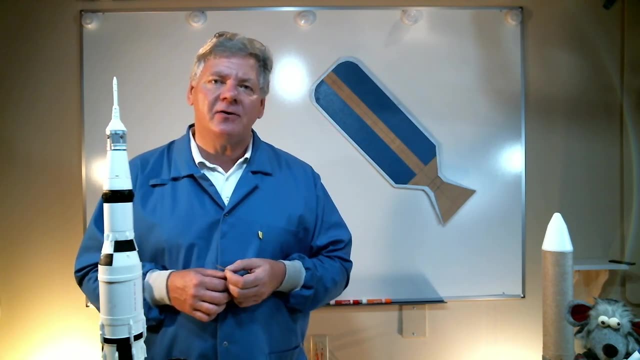 as a self-sustaining rocket motor igniter, except a NASA igniter produces a lot more heat and a lot more pressure to ignite a much larger rocket motor. So now let's take a look and experiment to see how a model rocket igniter works. 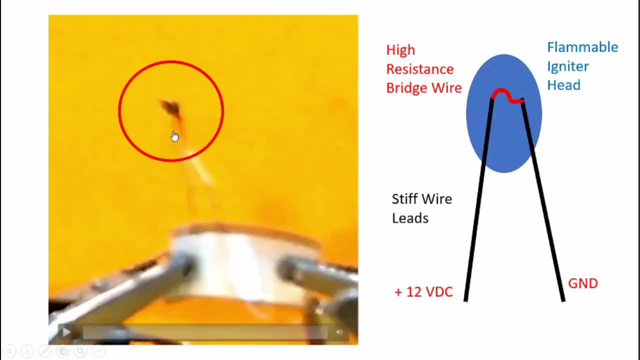 Here's the igniter. it's a model rocket igniter And this is a little graphic of what it looks like. We have the wire leads that lead to the firing lines of the ignition system, and those are depicted here. This blue represents a pyrogen-type material that burns the propellant. 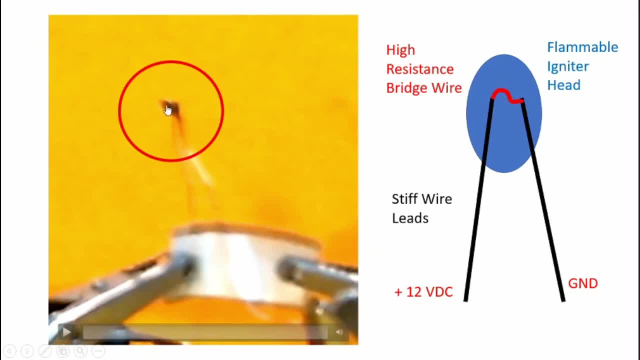 burns once it's subjected to heat, and that is this material here- And we have a small bridge wire, which is a high-resistance wire that heats up when current is passed through it. Again, that's what initiates the igniter. Now, what we'll do is we'll run the test and 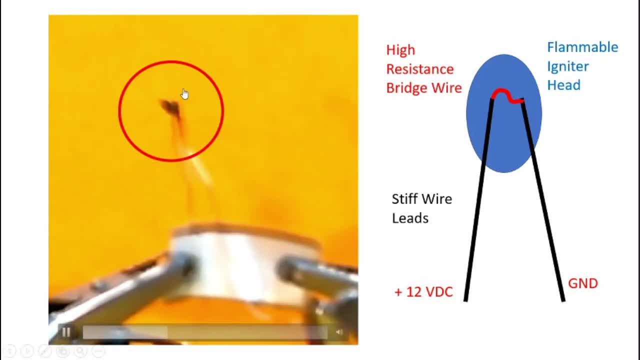 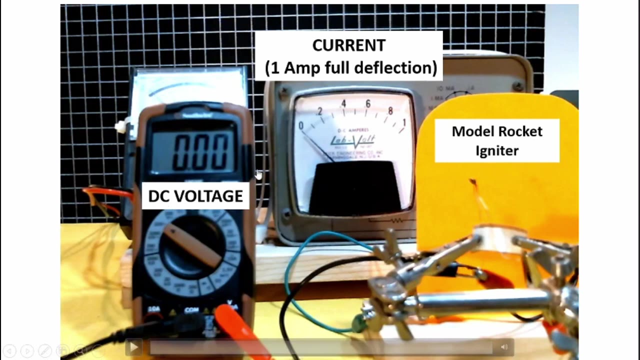 as we apply current and voltage to the igniter. eventually, once the current and voltage is high enough, we'll see the igniter go off. And there you have it. Now let's take a look at the test setup we used. Here's a test setup for our igniter test. What I have is a digital voltmeter here reading: 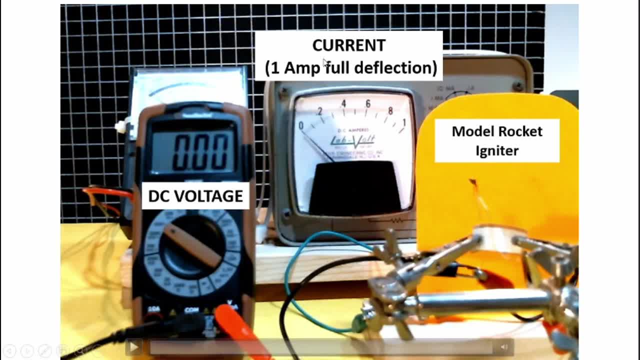 the voltage of the power supply. I've got a current meter reading. the amount of current passing through the igniter Full-scale deflection is 1 amp. so we have 0.1,, 0.2,, 0.3, 0.4 amps. 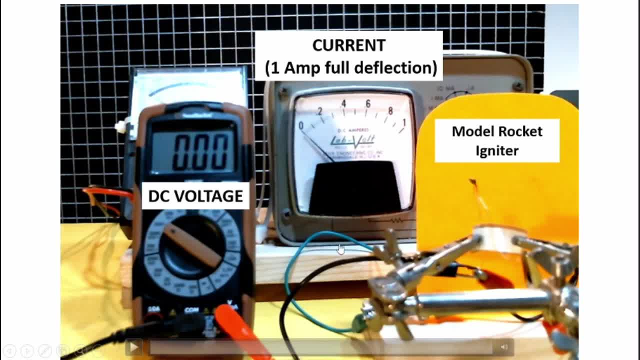 and so on. And here's a model rocket igniter. Now let's run the test and see what happens. We want to watch the voltage and the current. So what you see is a small increase in the voltage. Now let's run the test and see what happens. We want to watch the voltage and the current. 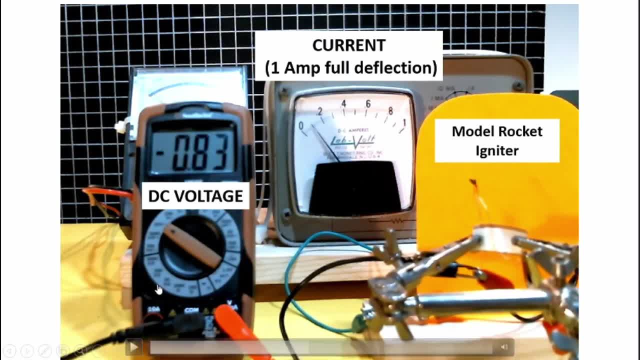 So what you see is small increases in the voltage. You'll see the current go up, and here you see, the current is at 0.1 amps, but the igniter still has not gone off and we're running about 0.83 volts Now because there's a closed. 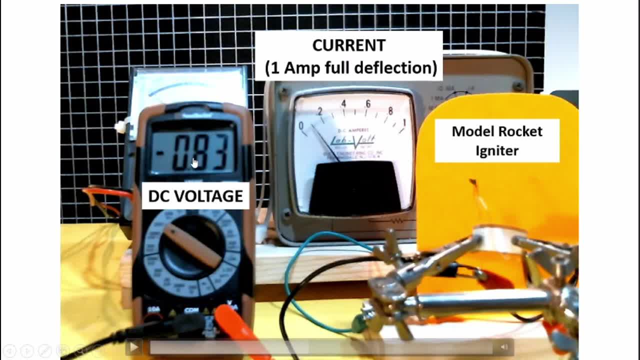 circuit in here. with the igniter it's actually drawing down the power supply, so the actual voltage being supplied to the igniter is greater than 0.83 volts, and we'll see that in a moment. So as we run the test a little bit longer, we see that the igniter burns, and it was. 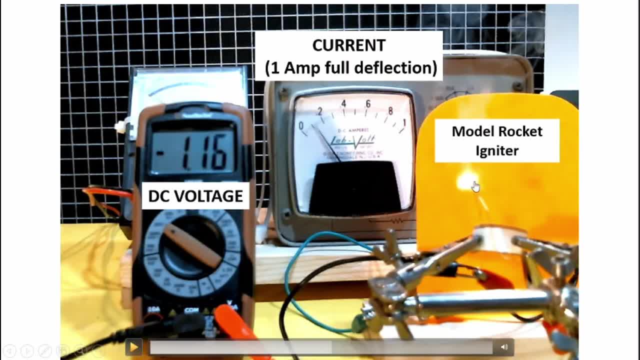 roughly 0.15 volts. Now, as the igniter burns, the resistance changes so the current drops and the voltage starts changing. So we run a little bit further. you can see that the current has dropped down to nearly 0, the igniter's burned and it's broken to open circuit. so we're actually seeing the 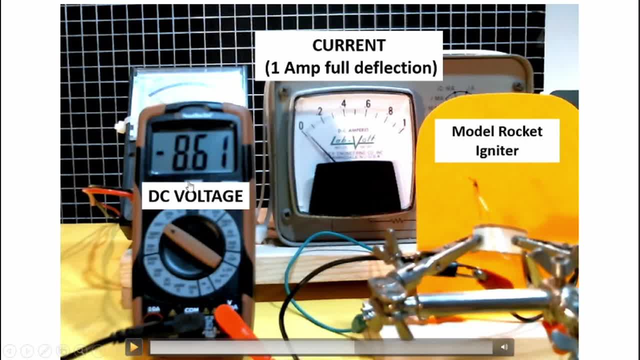 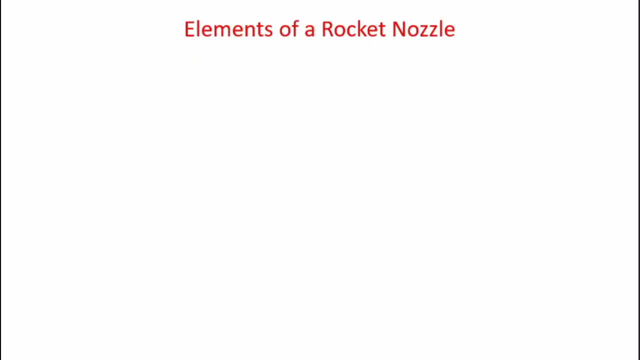 voltage of the power supply, and it's 8.61 volts. so that's the voltage required to get the igniter to burn, and we're required about 0.15 amps of current to ignite the igniter. So now let's take a look at the elements of a rocket nozzle. 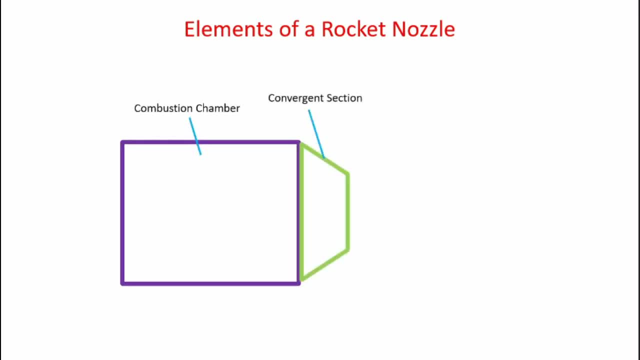 First of all we have the combustion chamber. Next we have a convergence section. Now in the convergence section, the cross-sectional area of the nozzle decreases as we move towards the right. Next is the throat. It's a constant cross-sectional area in the narrowest part of the nozzle. 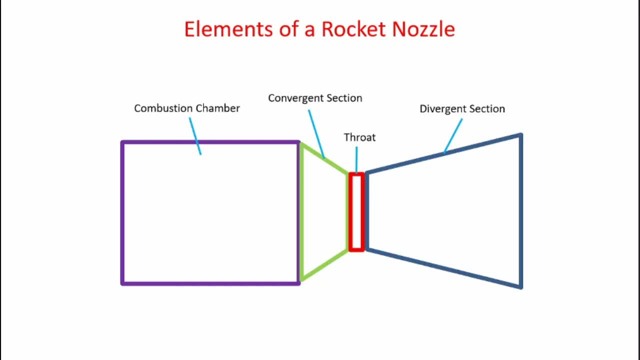 And finally, we have a divergence section. This is also known as the exit cone. And finally, we have a divergent section. This is also known as the exit cone. So let's take a look at the gas flow in the rocket nozzle. 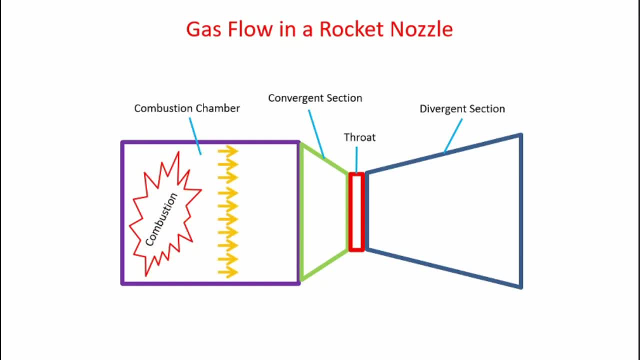 First of all, we have the combustion process taking place, which produces high-pressure gas that wants to move from the area of high pressure in the motor to an area of low pressure outside the motor. Now, this flow is subsonic. The velocity is less than the speed of sound. 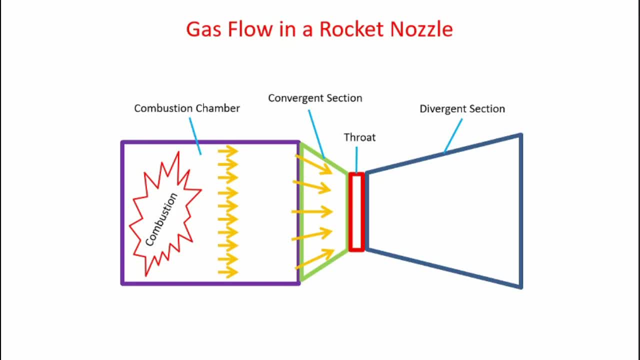 Now, when that occurs, when we decrease the area in the convergence section, the flow velocity increases, just like putting your thumb over the end of a hose and getting the water to squirt out faster. Now the goal is to get Mach 1 at the throat. 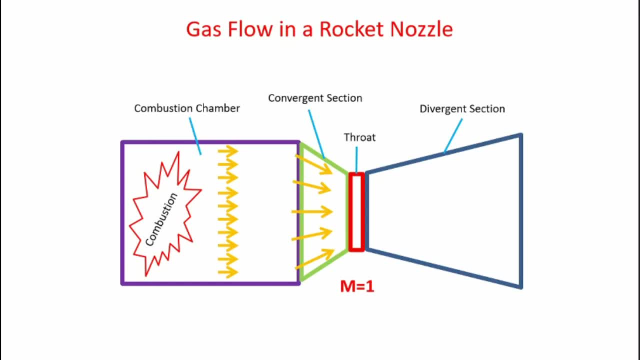 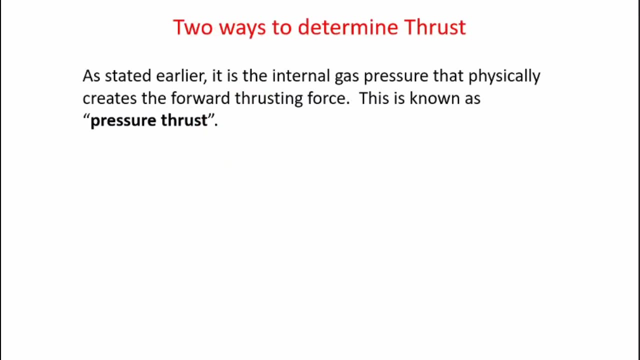 Now, when that occurs, we get supersonic flow in a divergent section. As we move towards the area of lower pressure outside the nozzle, the flow velocity actually increases, thus maximizing the exit velocity of the gases leaving the rocket motor. Now there are two ways to determine thrust. 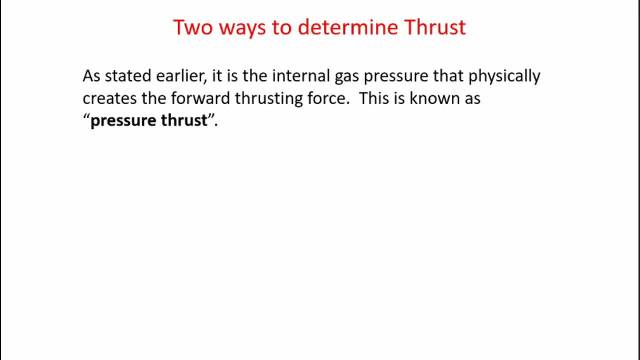 As stated earlier, it's the internal gas pressure that physically creates the forward thrusting force. This is known as a pressure thrust. However, thrust can also be determined by multiplying the mass flow rate- amount of mass flowing per second out of the motor- by the velocity of the gas, and we get momentum. 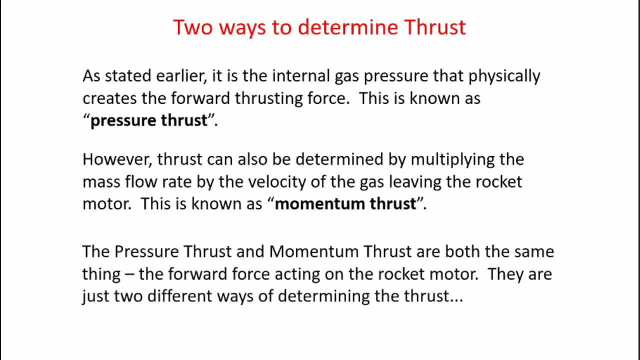 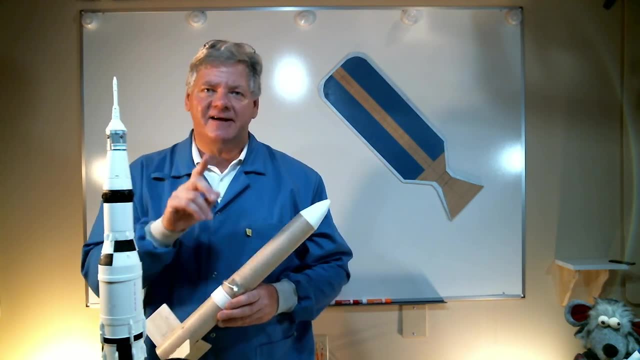 thrust. Now the pressure thrust and momentum thrust are both the same thing: the forward force acting on the rocket motor. They're just two different ways to determine the thrust. Well, that's the high-level basics of rocket motor thrust production. Now there's one more facet I want to talk about, and that's the thrust curve. 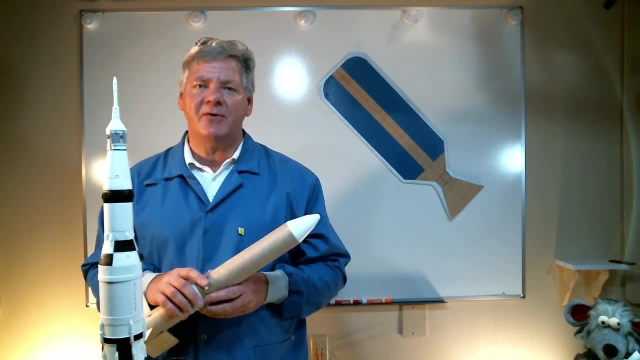 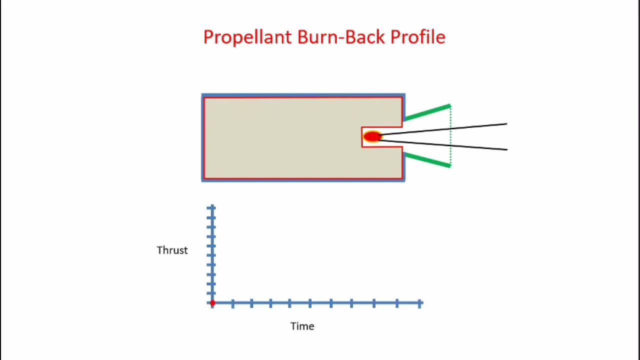 The thrust curve is the time-varying thrust level produced by the rocket motor. That information is critical to be able to predict the flight performance of a rocket. So now let's take a look at what's happening inside the rocket motor as the propellant 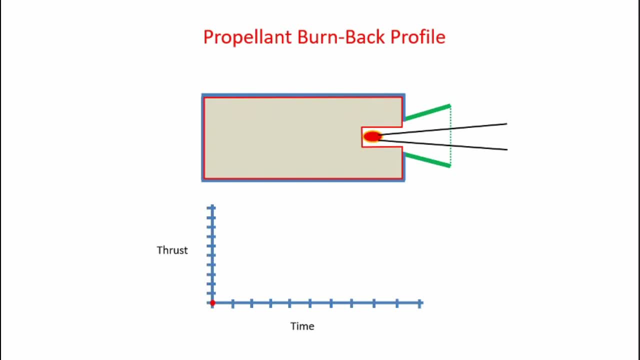 burns. In my simple little graphic I have an igniter depicted in red with the black leads and the red outlined area is the propellant inside the motor casing. At the bottom I have a graph of the propellant. The propellant burns. 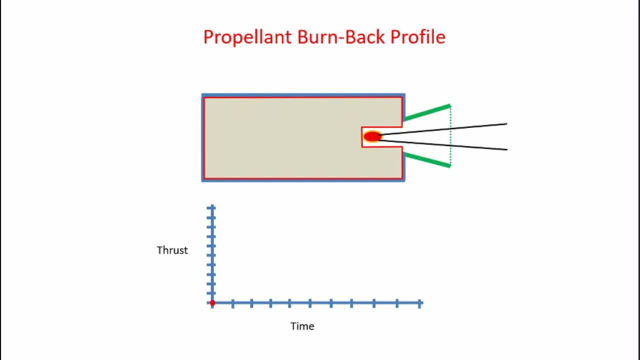 I have a graph which is thrust on the vertical axis and time on the horizontal axis. Now, when I apply current to the igniter, it begins to burn and it in turn ignites the surface of the propellant. Now, initially the propellant burns outward, towards the casing wall and forward and as. 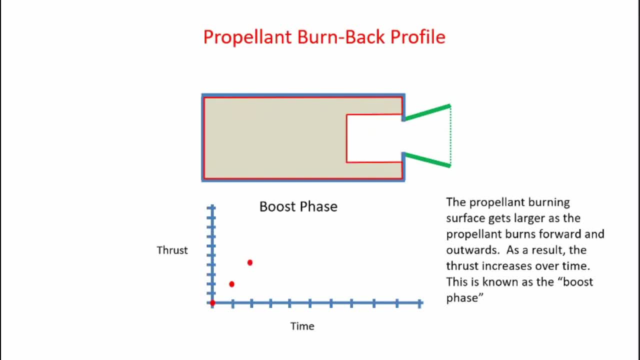 it does, the burning surface area increases. This increases the pressure inside the rocket motor and also increases the thrust Again. the surface area increases as it burns Until eventually it burns to the casing wall. Now the surface area drastically drops at this point and the thrust drops off as well. 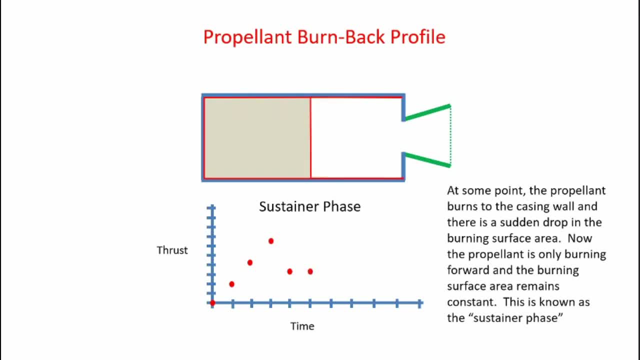 You can see that in the points on the thrust curve. Then the motor burns from the end towards the front of the motor. This is known as the sustainer phase of the motor burn. Eventually the propellant burns out to the forward end of the casing and the thrust 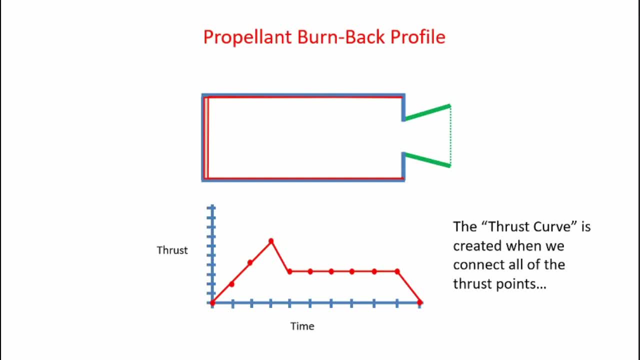 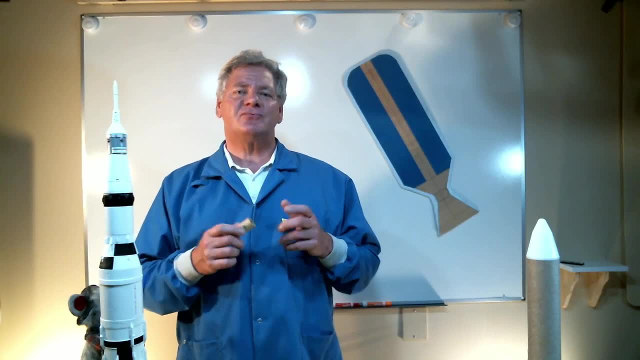 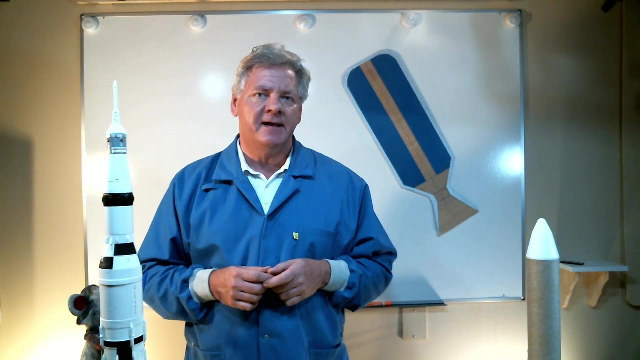 drops to zero. Now, when I connect these points with a line, this creates the thrust curve, which is thrust versus time. Okay, so let's wrap things up with a static firing of a C-65 model rocket motor. Now, the first view we'll see is in real time, and the second view we'll see is in slow motion.